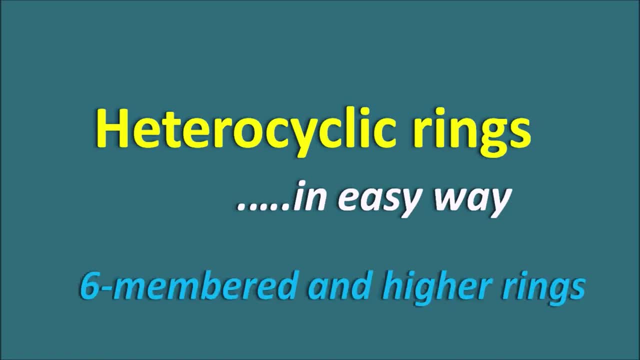 Hi, today we will discuss six membered and higher heterocyclic rings in easy way. In our previous video we have discussed the three membered to the five membered heterocyclic ring systems and what is their nomenclature, And today we will discuss the six membered and higher ring systems and what is the nomenclature and how we can give the numbering to these heterocyclic ring systems. 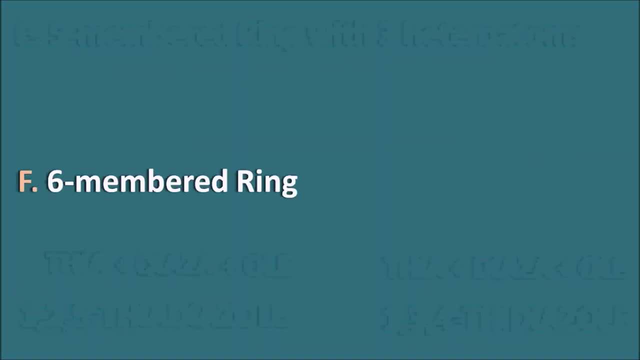 Now let us go with the six membered ring systems. So the simple ring system is the six membered ring system with one heteroatom as the nitrogen. So all we have seen this is the pyridine. So pyridine is the nitrogen containing six membered ring system. 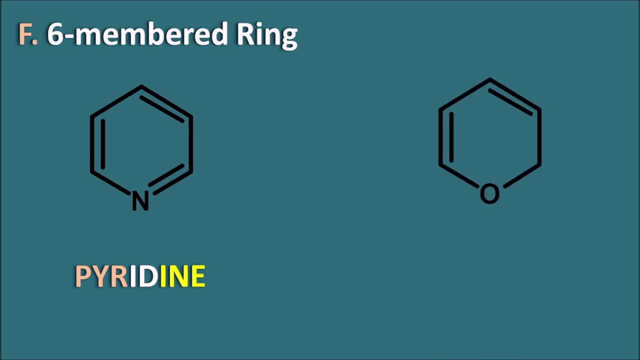 And if it is auxin is present, then it is called as pyrone. But in this pyrone second position is saturated because auxin is having the valency as only two. So the second position should be saturated. So here we are going to indicate the point of saturation with its position and the letter H. So 2H indicates second position is saturated. So this is a 2H pyrone. Again, here we are not following any particular suffix. So they should be well known with their common names, like the pyridine and pyrone. 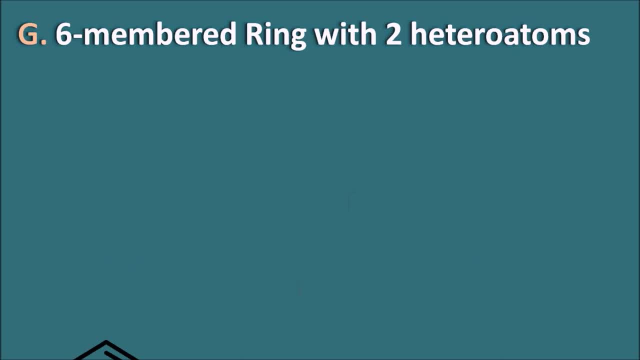 Now the six membered ring systems with two heteroatoms. Now here we can add another heteroatom, nitrogen, at the second position. Otherwise we can add the another heteroatom at the third position And finally we can also add this heteroatom at the fourth position. So nitrosines can be present at the first and second position, or first and third position, or first and fourth positions. 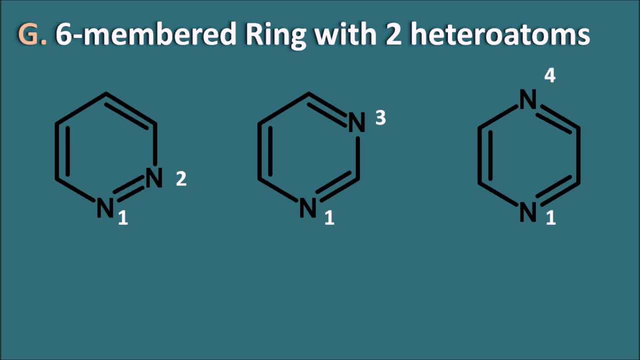 Now, how can we write the name for these ring systems Here? the first one is coming from the pyridine and an extra nitrogen is there, like the EZA, just like in the pyrozole, which is a five membered ring system. Here we can apply the same logic. So pyridine within the pyridine, we are going to introduce the EZA. 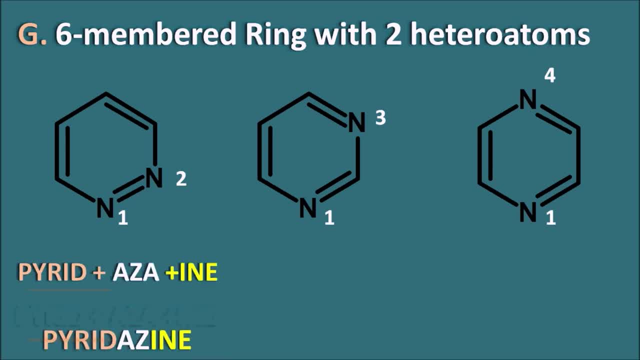 So Pyrid plus Azar plus Ein, so that is a pyridazine. If you remove the Az, it's simply pyridine. So within the pyridine we have introduced the Azar because it's having an extra nitrogen. 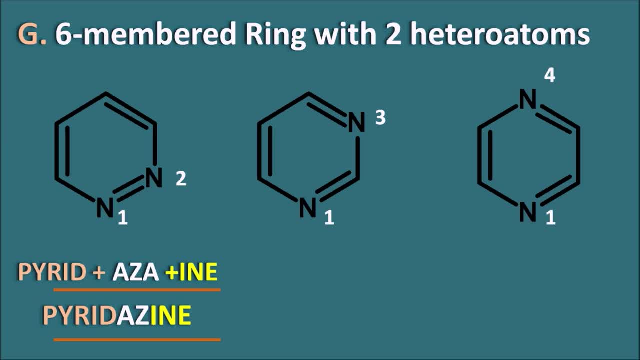 at the adjacent position. So that is a pyridazine. And what about the second one? So, just like the previous, imidazole, so here pyr plus imid. imid indicates that is a meta position, that is a third position and is a six member ring system. that is the Ein, as. 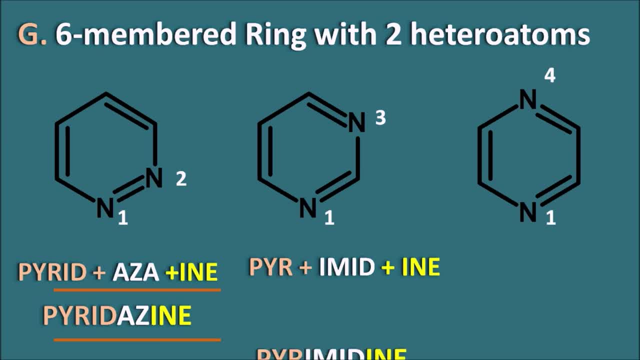 a suffix. So pyr plus imid plus Ein. so this is the pyrimidine. So pyrimidine is having the nitrogen at the first and third positions, And what is the name for the last one? Here the one of the nitrogen can be indicated as a pyr and then the nitrogen as the Azar. 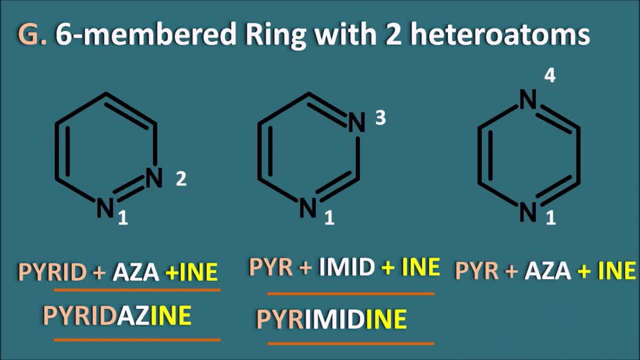 and suffix as Ein. So pyr plus Azar plus Ein, that is the pyridazine. So here we have to remember that in the pyridazine nitrogen is present at the second position. so we have written the pyrid, But in the pyridazine it is present at the second position. 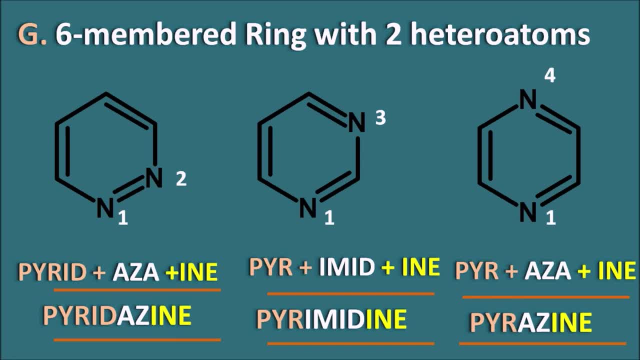 So pyridazine is present at the second position, So pyridazine is present at the fourth position. we have taken only prefix pyr, So pyridazine is one two and pyridazine is one four. So here we have three types of heterocyclic ring systems with two heteroatoms. 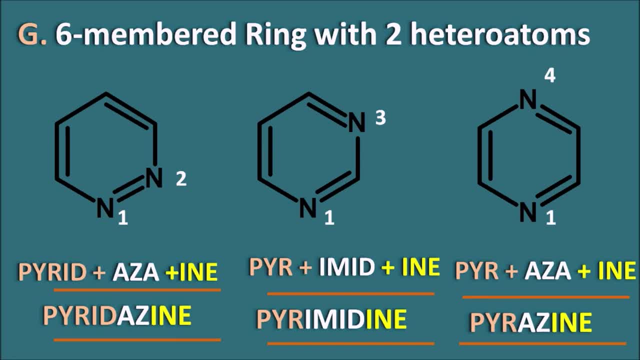 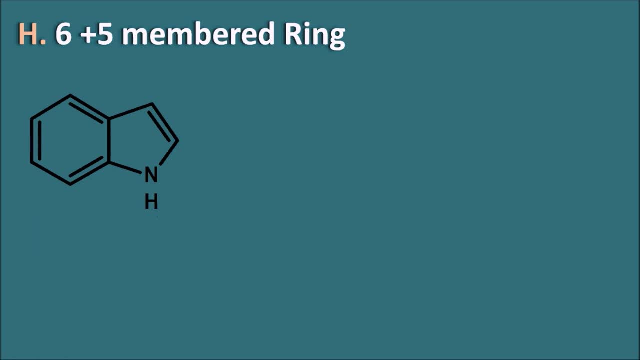 So pyridazine, pyrimidine and pyridazine. Now let us go with the six plus five member ring systems. So this is the one of the six plus five member ring system. the six member ring system is the simple benzene and second one is the heterocyclic ring system, which can be called as pyrrole. 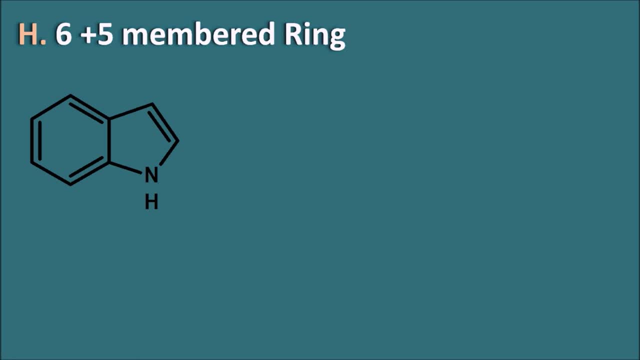 So simply it can be written as benzene. So the benzo pyrrole. but actually this ring system is commonly known as indole. So indole is a six plus five member ring system with nitrogen as the heteroatom. Similarly, another one is the benzene with furon. 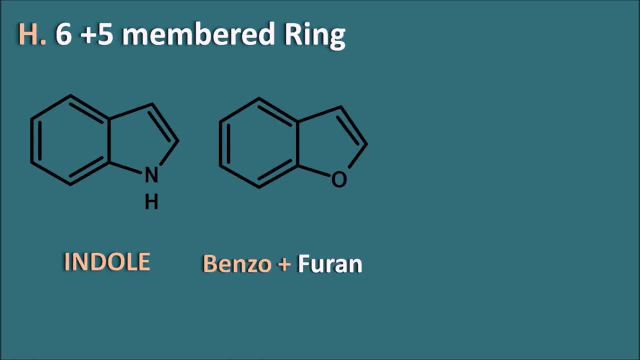 When the benzene is gone to be fused, it can be written as benzo plus furon, So it is benze, furon. Similarly, this structure benzo plus thiophene. this is the benzothiophene. These names can be directly derived by using the whatever this term: benzo. 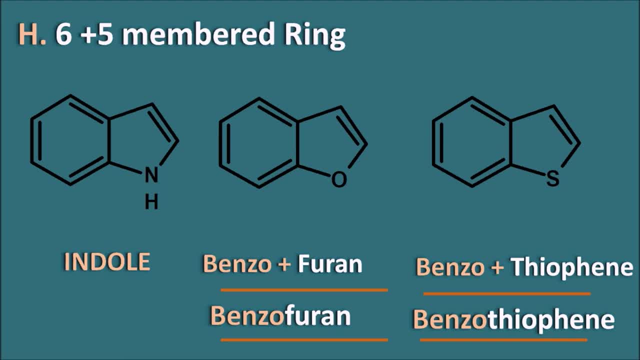 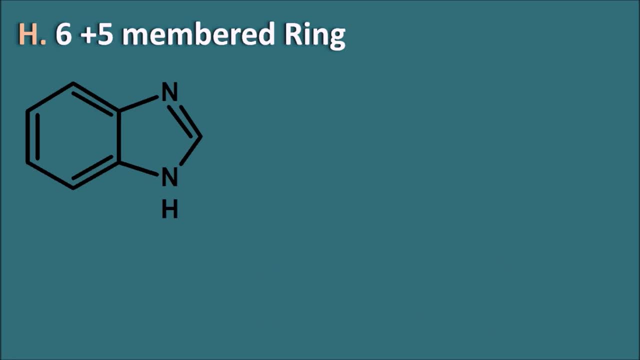 when the benzene is going to be fused with the heterocyclic ring systems. Now let us take another example with the 6 plus 5 member ring system, with two heteroatoms here. So what is the name of this one? So now here the what are? the heterocyclic ring system is the. 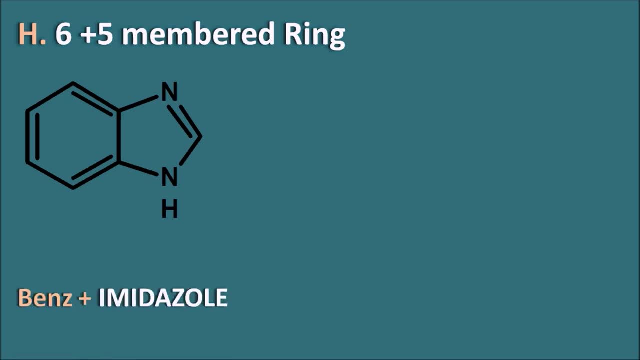 imidazole, which is attached with the benzene. So benz plus imidazole, that is the benzimidazole. So here we have not used the O because it is not easy to pronounce, So benzimidazole is simplified as benzimidazole. Similarly, another one is the benzene with the oxazole. Now here this is the. 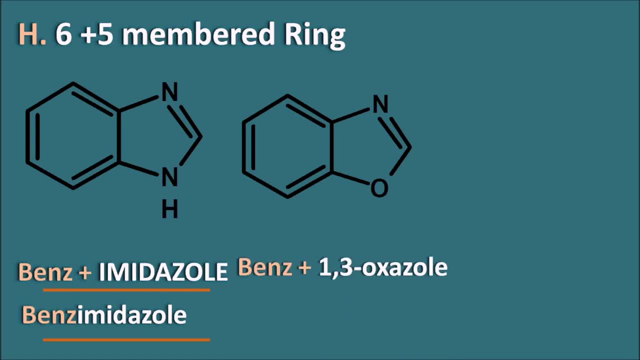 benz plus 1,3-oxazole, So that is the 1,3-benzoxazole. Similarly, third structure with the sulfur. So again here, benz plus 1,3-thiazole, that is the 1,3-benzothiazole. Now let us go with the. 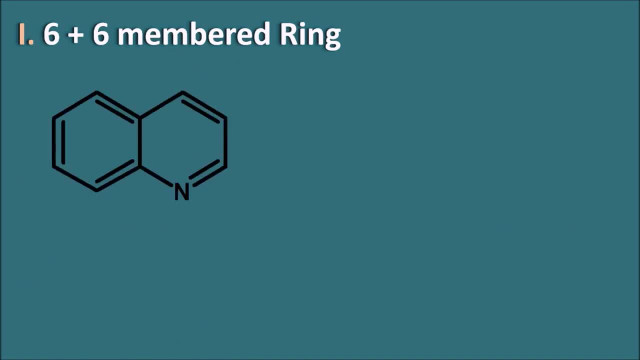 6 plus 6 member ring systems. So this is the one of the 6 plus 6 member ring systems. So this is the one of the 6 member ring system with having nitrogen. So again, this heterocyclic ring system is commonly known as quinoline, So here the nitrogen is present at the first position. 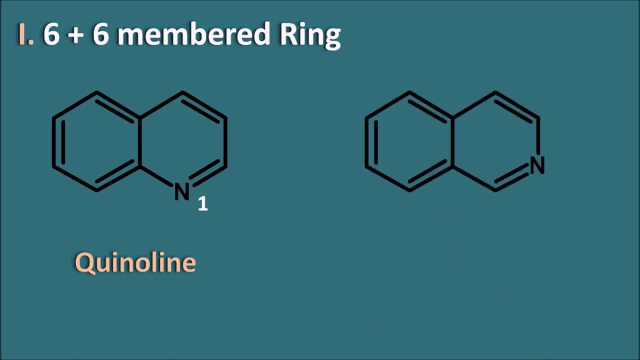 If, suppose, if position of the nitrogen is going to be changed like this: Now, here the nitrogen is present at the second position, So this is called as isoquinoline, So quinoline and isoquinoline. Quinoline is one of the important ring system in present in the anti-malarials like 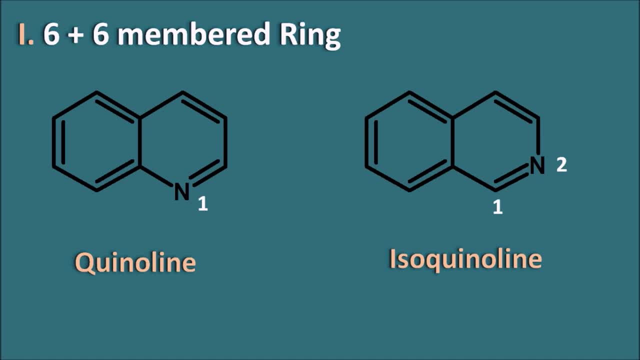 the chloroquine, mefloquine And isoquinoline is one of the important ring systems present in the anti-malarials like the chloroquine, mefloquine And isoquinoline is one of the important ring system present in the smooth muscle relaxant like the papaverine. 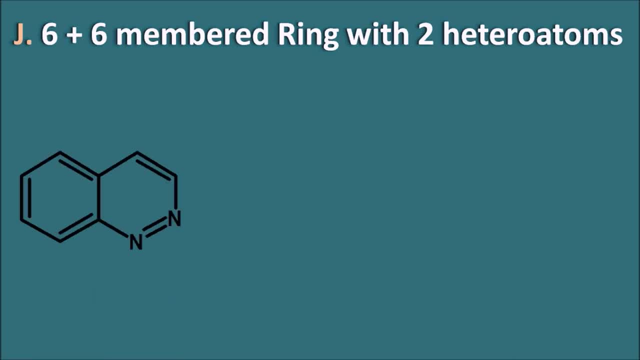 Now 6 plus 6 member ring system with two heteroatoms. So this is the one of the ring system. So this is the one ring where the nitrosines are present at the first and second position. This ring is commonly known as synoline, And the nitrosines can also be present at the 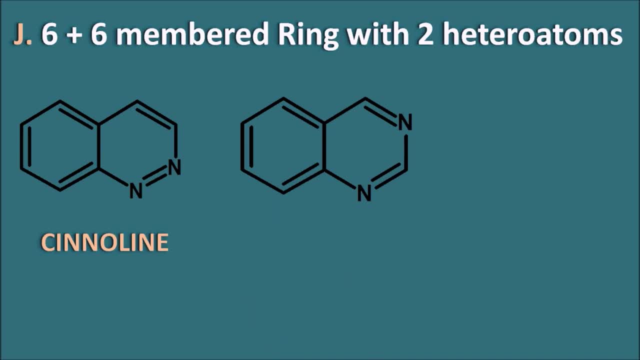 first and third position, Then this name of this ring can be derived from the base name quinoline. So because if single nitrogen is present, that is quinoline. So quinoline plus extra nitrogen as aza, that is quinazoline. Similarly, if the nitrogen is present at the first and fourth position, then 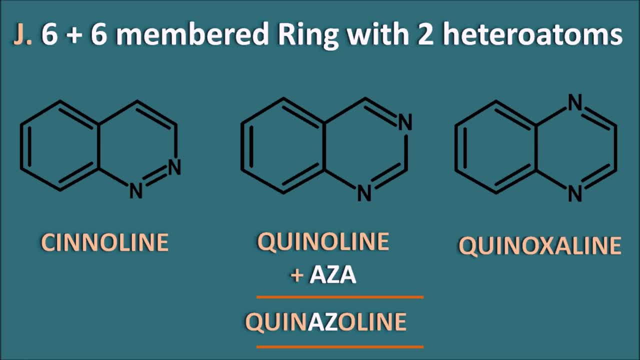 it is commonly known as quinoxaline. Here don't think that OX indicates oxygen is present. This ring is commonly known as quinoxaline, where the nitrosines are present at the first and fourth positions. These rings are well known with their common names. we have to remember as it is. 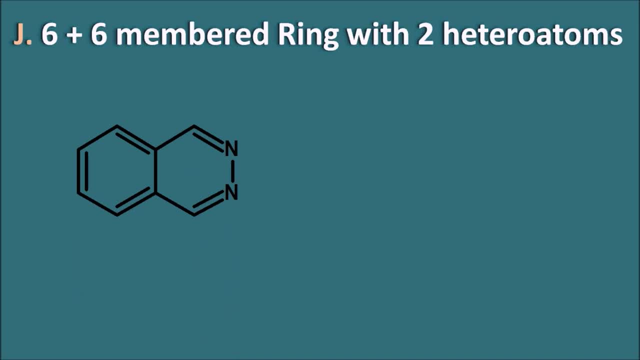 The next one is the ender heterocyclic ring system. But here you can observe that the nitrosines are not present at the first position. So if we give the name ring here this is one, two, three and four. That means here the nitrosines are present at second and third positions. 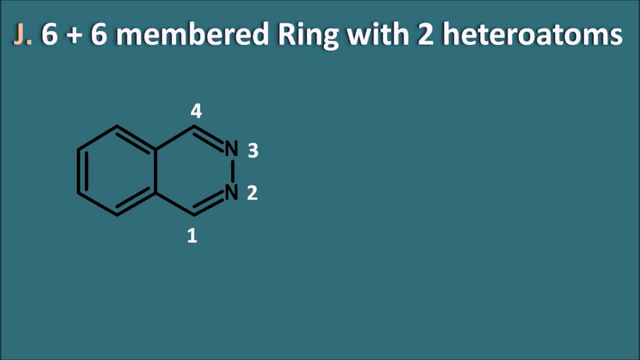 How we can give the name for this compound. So if we compare this ring with the aromatic ring system having two rings, so this is nothing but simply naphthalene. So from the naphthalene we can derive a small part which can be used for the naming of this heterocyclic ring system. 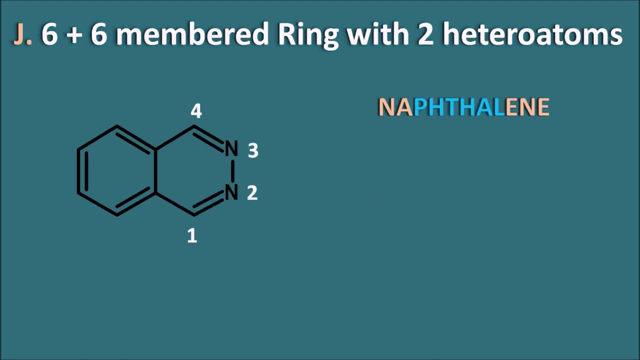 can take the phthal as one of the part. So from the naphthalene we can take the phthal and since the nitrogen is present, we can use the aza. but here we are not using the diaza. even two nitrons are present. simply, we are indicating the nitrogens which are going to replace the carbon as the aza. 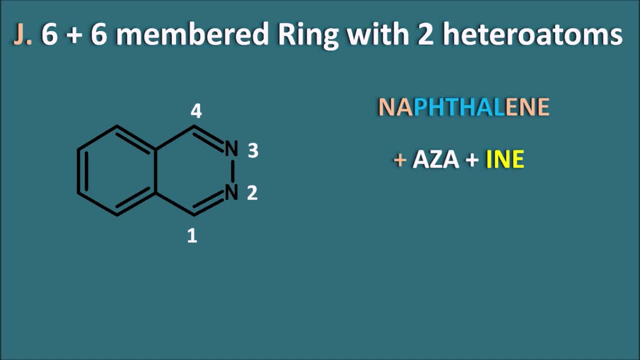 and the nitrogens are present in the six member ring system. so ein, so what are? the complete name is the phthalozyne. So here we are going to discuss like this in order to remember very easily, because in the six plus six member ring system the two nitrogens can be present at the first and 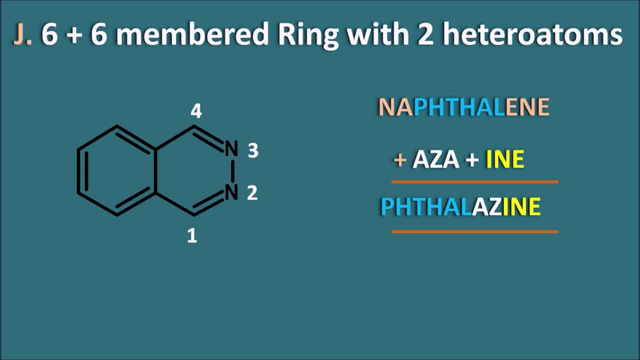 second position, first and third portion and first and fourth position as well, as they can also present at the second and third position. So when they are present at the second and third position, we can simply compare it with the naphthalene and from that we can derive the name, so the 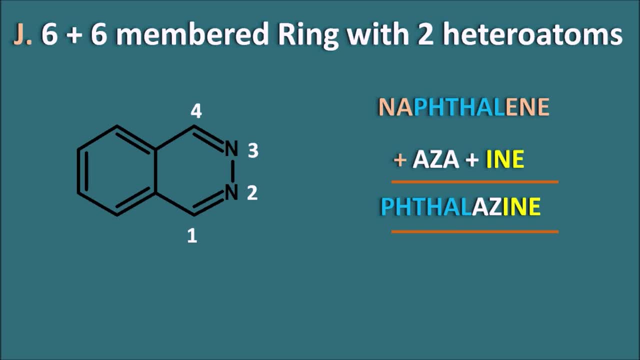 whatever, this heterocyclic ring system is derived from the naphthalene ring and the name is the phthalozyne. This phthalozyne ring is present in one of the drug. hydrologyne. hydrogen is a vasodilator used to treat the hypertension, as well as in the treatment of 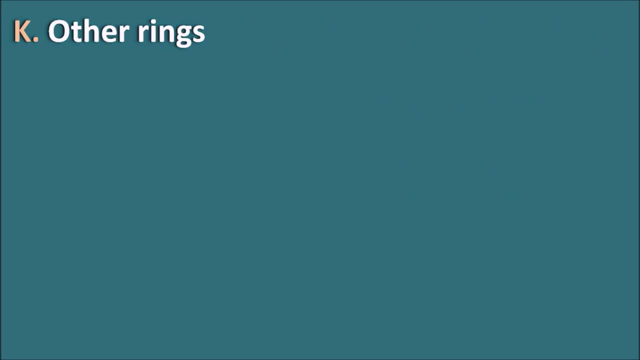 alopecia. Next let us go with the other rings. so now this is a ring of six plus seven member ring system. and here you can observe it is hanged again two heteroatoms, that is, the nitrogens. So from which position we have to give the numbering? always in the compounds hang two or more. 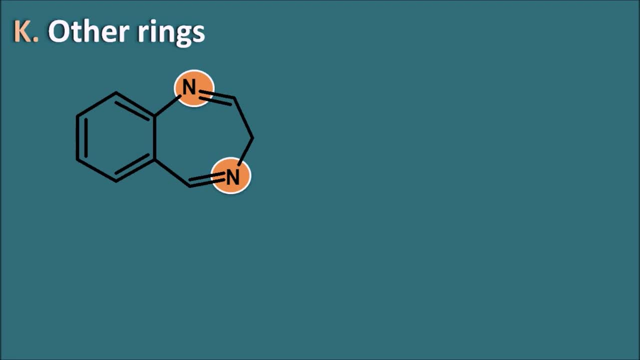 rings. we have to give the numbering from the atom adds into the bridge heads. so we can give the numbering either from the bridge heads or from the hydrogens. so we can give the numbering either from this atom or from this atom which are ads into the bridge heads. bridge heads are nothing but what. 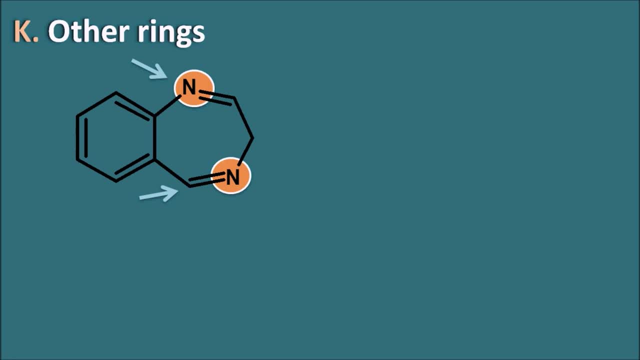 are the atoms which are which are involved in the fusion between the two rings. so we can start the numbering from any of these atoms. but if we start the numbering from this nitrogen- one, two, three, four, five- we can give the lowest number to the both of the nitrogen. so this numbering is correct. 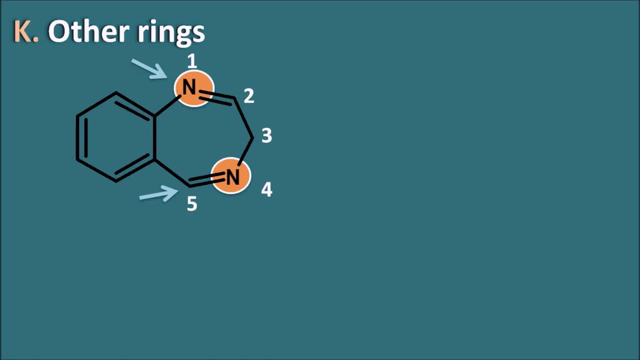 so nitrons are present at first and fourth positions, and here you can observe that the third position is saturated. it is not attached with any double bond, So which we can indicate with an indicated hydrogen 3H. so if we give the name, this is 3H plus benzo, because benzene is going to be fused benzo. 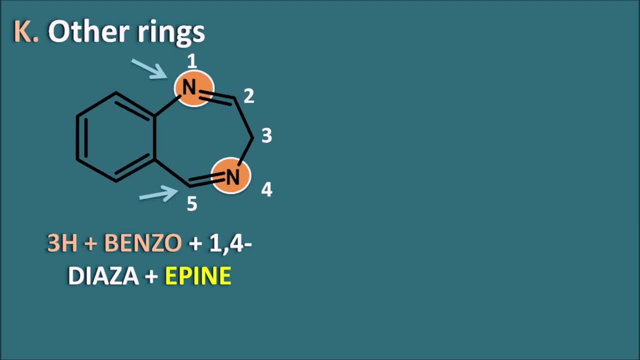 and nitrogens are present at the first and fourth position. so one four diaza, and this is a seven member ring system with nitrogen. so whatever the suffix is the epine. so by combining all these we can get the name as 3H- benzo digepine or 3H- one four benzo digepine. 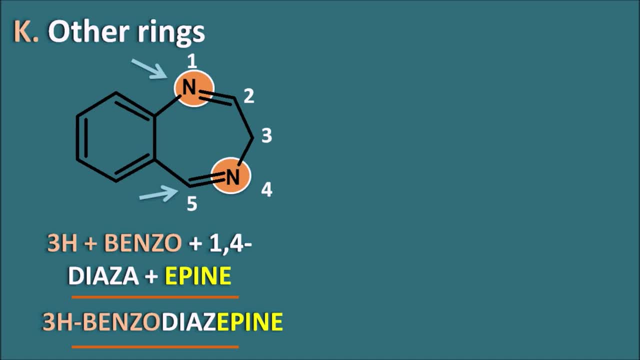 simply we can write benzo digepine, because most of the benzodiazepines are having the nitrogens at first and fourth position. so this is the 3H one, four, benzo digepine. similarly we can go with the another ring where here it is saying the sulfur and nitrogen. so we can start the numbering. 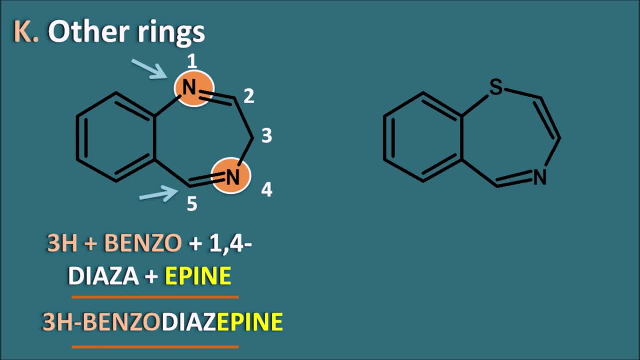 from the sulfur, because sulfur should be given more preference than the nitrogen. so this is one, two, three, four and five. so just like the previous one, but here there is no saturation point. so simply we can write: benzo, benzo digepine, plus one four diaza plus epine. so that is the one four, benzo digepine. or simply we can write: 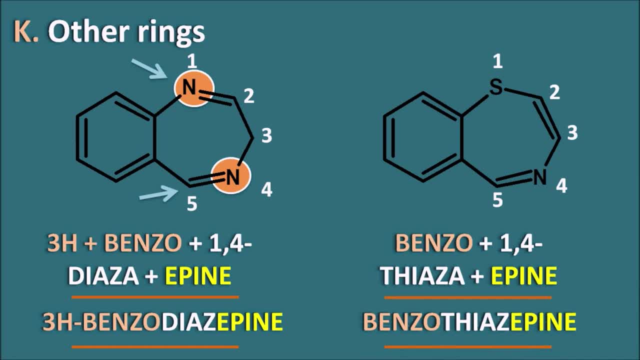 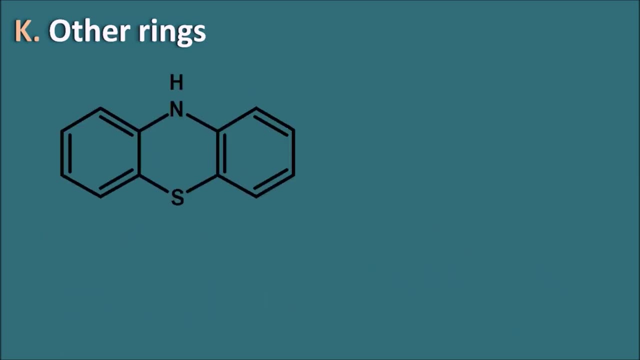 benzo digepine, but it should be indicated as one four benzo digepine, because we also have one five benzo digepine. so in order to differentiate we have to indicate it with the one four. so the water, the ring system, is the benzo digepine, similarly another one. here you can see the three. 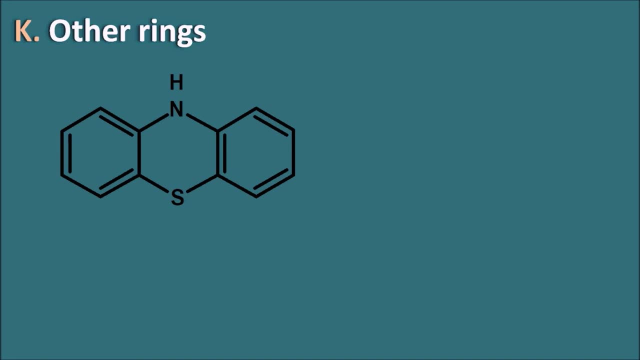 rings are there. so it is a tricyclic ring system. so from which atom we have to give the numbering? here sulfur should be given the least number. but we cannot start the numbering from the sulfur because sulfur is there in the middle ring. we cannot start the numbering from middle of the ring. we should start the numbering from any of the terminal. 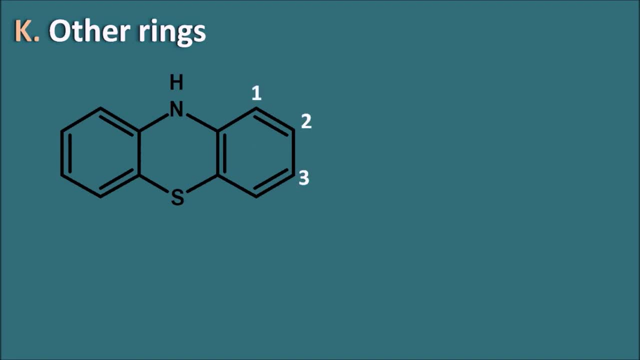 so let us start here. this is one, two, three, four and five. so in this way we have given the least number to the sulfur, that is, five. if we try to give the numbering in reverse direction, sulfur will get the more number, which is not correct. sulfur is given the fifth number, then six, seven, eight, nine and ten. so now the sulfur is present. 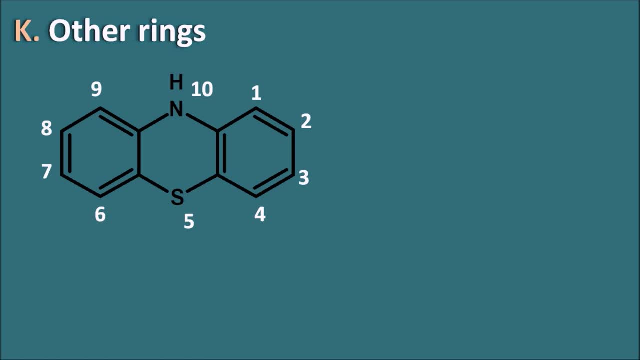 at the fifth portion and nitrogen is present at the tenth portion, and because the nitrogen is saturated here we can indicate this as 10 h, so 10 h plus pheno. even here two phenyl groups are there, but here we are not using again diphenyl or diphenyl. simply we are going to indicate by: 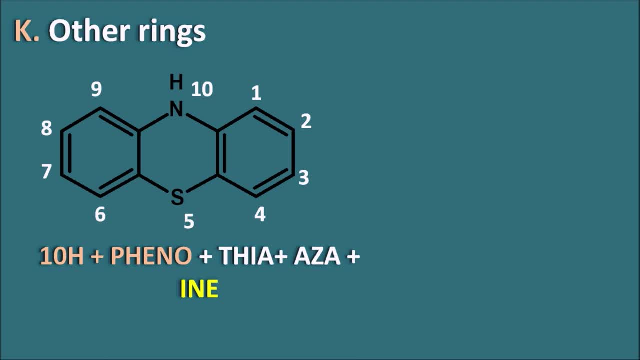 pheno. that means pheno indicates the pheno group is going to be flanked on both of the of this heterocyclic ring system. so 10 h plus pheno plus sulfur is indicated by thia and nitrogen is indicated by aza, and sulfur and nitrogen are present within a six member ring system, so the 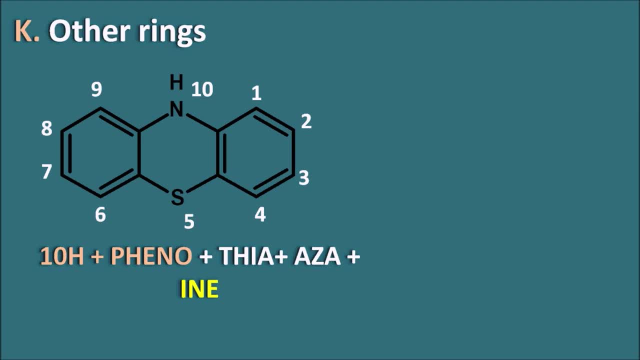 suffix. is i combining all these, we will get 10 h phenothiagine. so phenothiagine ring system is present in the well-known drugs which are used as the antipsychotics, like chlorpromzine, triflu, promzine, flu, phenazine. in all of these phenothiagine ring system is present. 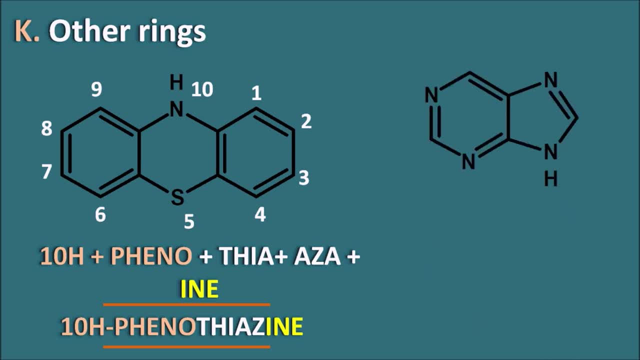 similarly, another heterocyclic ring with so many hetero atoms. here you can observe, four hetero atoms are there and the numbering is somewhat different in this ring system. this ring system is made up of two heterocyclic rings. one of the heterocyclic ring is made up of pyrimidine and another 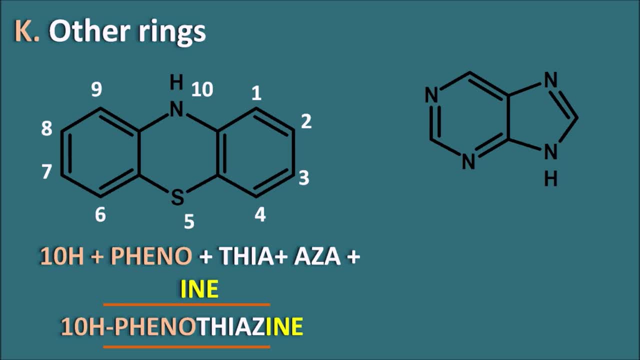 heterocyclic ring is the imidazole, so this is the imidazolo pyrimidine. but if we give the numbering here, so we have to start the numbering from the pyrimidine ring. so one, two, three, four, and here you can see that we are giving numbering even to the bridged heads in the previous examples. 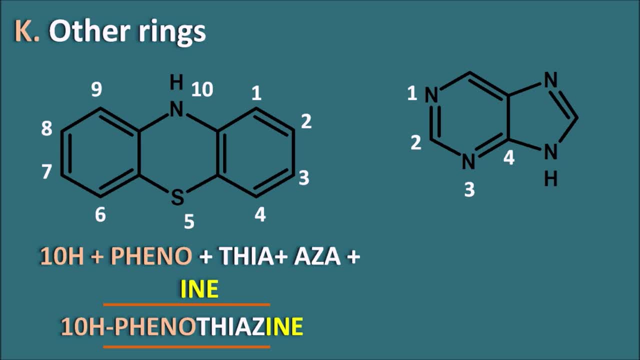 we are not giving the numbering to the water of the bridged heads, but in this structure we will give the numbering to the bridged heads. so four, then we are giving the five and six. that means we are completing the numbering to the pyrimidine ring initially, then to the imidazole. we are going. 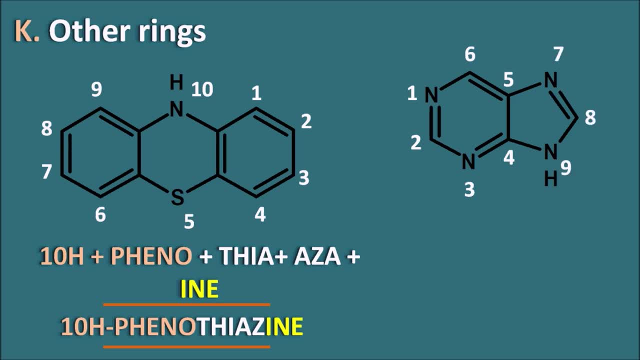 to continue there. so seven, eight and nine. so saturated nitrogen is indicated by ninth position. so this is commonly known as a purine ring, which can be indicated as 9h purine. so 9h purine is a imidazolo pyrimidine, but it is commonly known as purine ring system. in this way we can have: